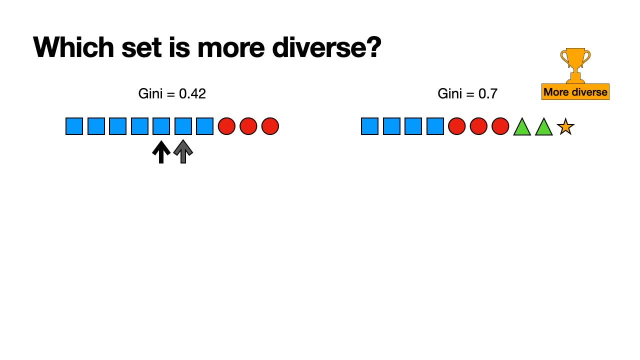 these two elements. Now I'm allowed to pick the same element twice. there's no restriction about that and also it's an ordered pair, So there's a first and a second that I pick. So if I pick these two and I look at the classes, they're both blue squares, So I record them and I record that. 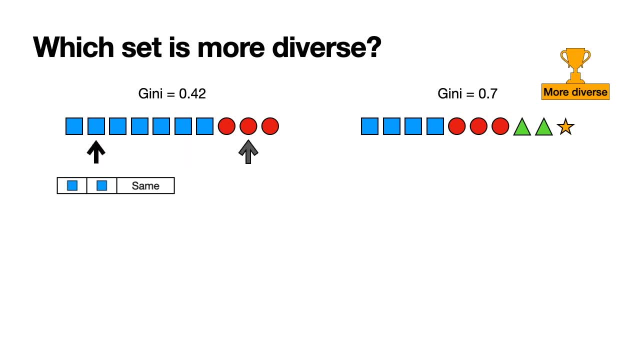 they're the same type of element. Then I do it again and I get blue square, red circle. and I do it again and I get red circle, blue square, And I continue doing this for a long time. So I'm going to do it 10 times And I'm going to record how many times did I get a different pair. 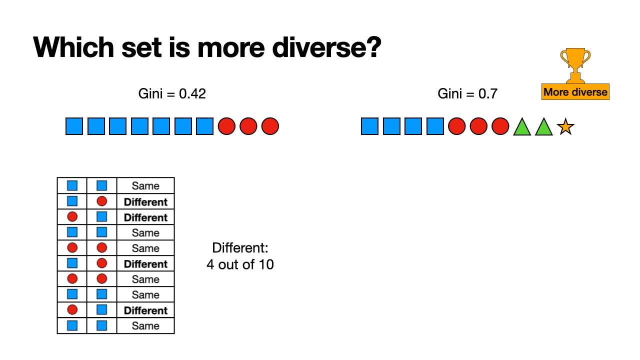 So it's 4 out of 10.. Now what does your intuition tell you? If I do this on the set on the left, then I'm going to get more distinct pairs or more equal pairs. So let's do it. I pick 10 random pairs. 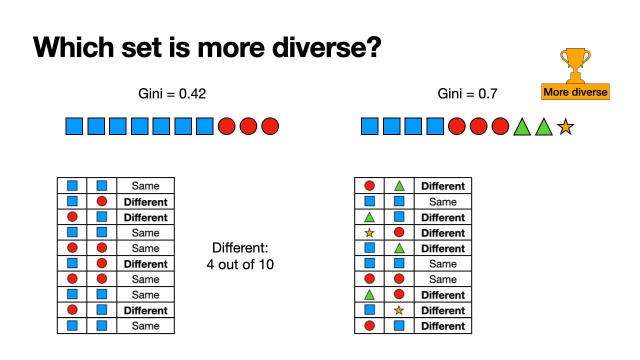 and I get that they're different. So I'm going to do it again and I get red circle, blue square different 7 out of 10 times. And this makes sense, right? Because the more diverse the data set, if I pick two random elements, I'm going to get two distinct classes more often in a diverse. 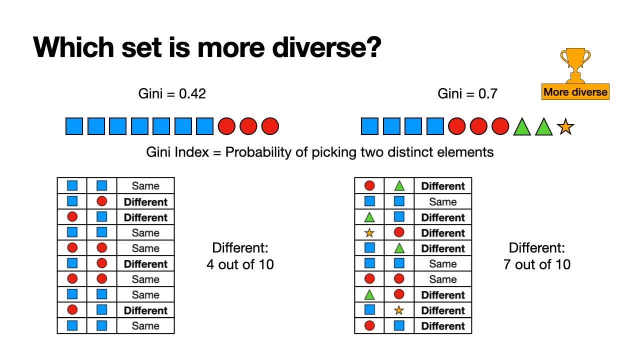 data set than in a non-diverse data set, And that's precisely the Gini Impurity Index. It's, if I take two elements out of my data set, an ordered pair. what is the probability that they're going to be of distinct classes? And that probability is the Gini Impurity Index And, as you can see, 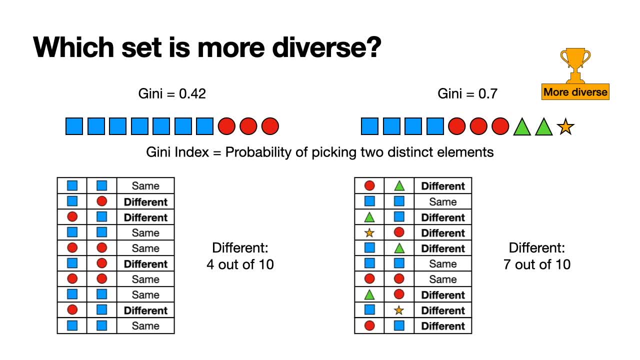 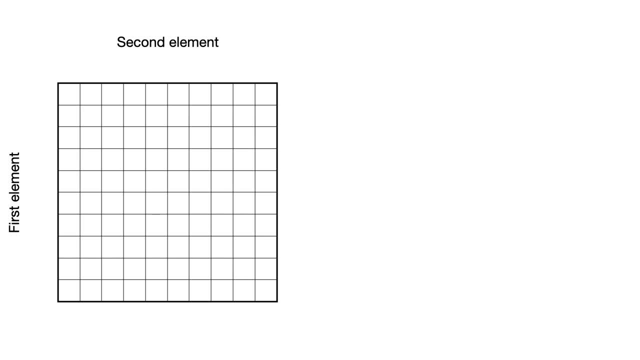 it's higher the more diverse a set is. So let's calculate this probability for these two data sets, And the way I like to calculate probabilities is by taking all the possibilities. So let's start by putting our 10 elements in the left part of a square and the same 10 elements in the top row of that same square And the square. 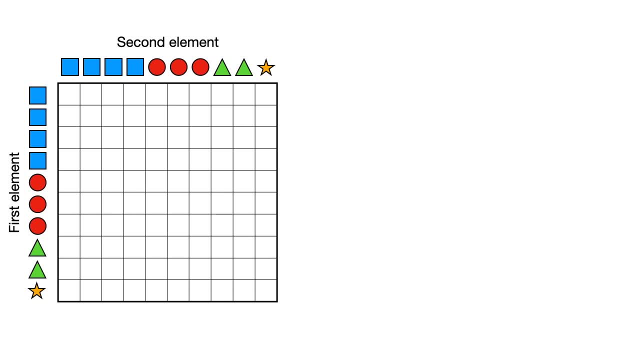 has 100 boxes because it's 10 by 10.. So all the pairs are recorded in the square. Here are where I take two squares, two blue squares. Here I take two red circles. Here's where I take two green triangles And here's where I take two yellow stars And I fill this in with all the 100. 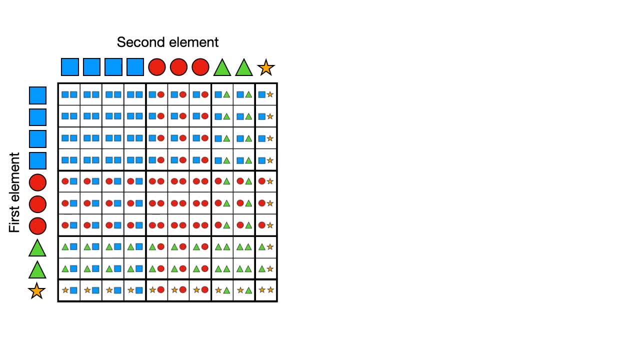 possibilities. So, as you can see, the ones where the two elements are equal are this blue square, this red square, this green square and this yellow square, And the ones where they're different is everything else. So what I want to do to calculate the probability that my two elements are distinct. 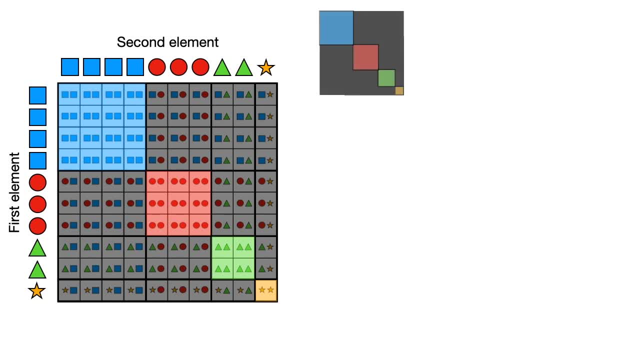 what I need to do is to calculate the black area. So I'm going to calculate the black area by doing this operation. I'm going to say that the black area is the big square minus the areas of the colored squares. The black area is the probability that the both elements that I pick are different. 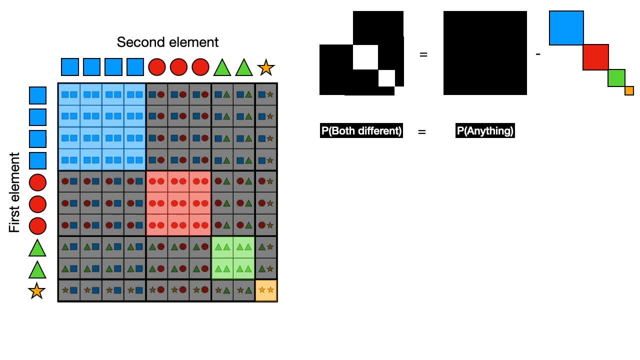 The whole square is anything, because it's the entire universe of possibilities, And then the rest is the probability that they're both equal. So the probability of anything is always one, because it has to happen, And then the probability of both equal is the sum of the. 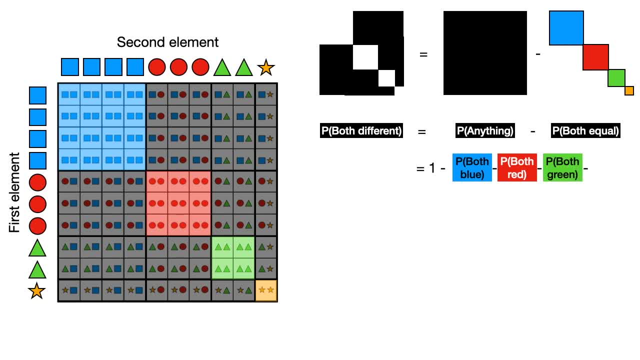 areas of the blue square, the red square, the green square and the yellow square, because it's precisely when they're both blue and they're both red, both green and both yellow, And now I need to calculate the areas of the blue square, the red square, the green square and the yellow square. 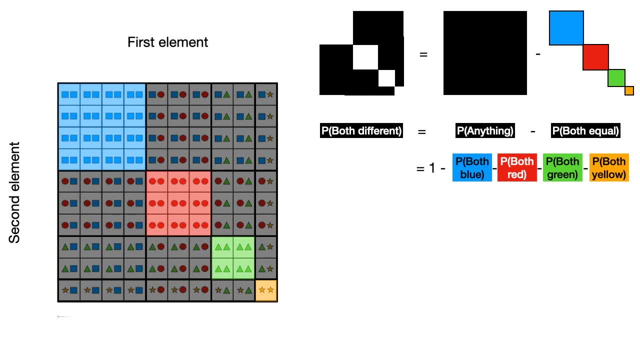 How do I calculate that? Well, let's look back at the square and say that it has a length, a base and a height of one. And so what are the proportions? Well, it's four tenths for the blue square. 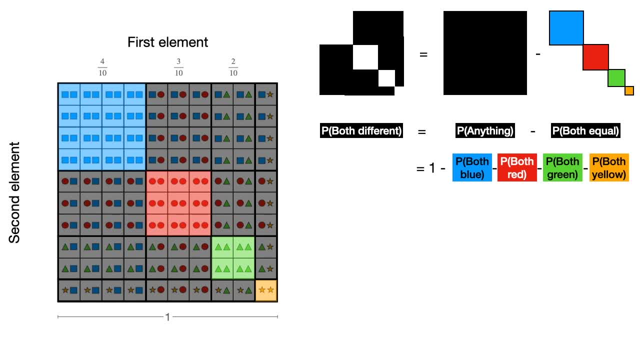 It's three tenths for the red circle, It's two tenths for the green triangle And it's one tenth for the yellow star, And the same thing along this edge. And so now I can calculate areas by multiplying the base times the height. So the blue square has area four tenths square The red square. 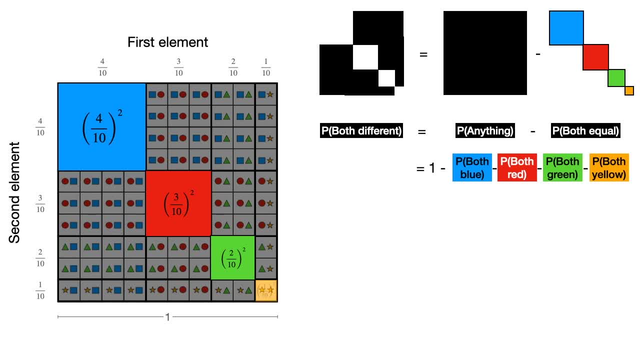 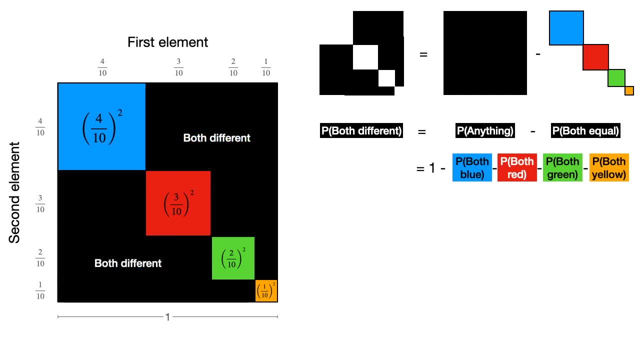 has area three tenths square, The green one has two tenths square And the yellow one has one tenth square of an area, As I mentioned before. for everything else, that area is the one that I want. So now let's calculate it. It's one minus four tenths square minus three tenths square minus two. 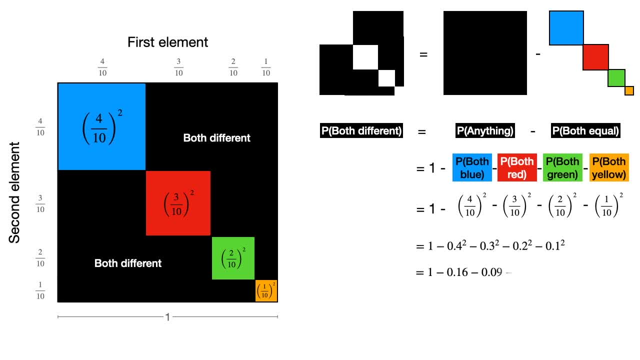 tenths square minus one tenths square, which I can do some math, And that's 0.70.. So 0.70 is the probability that I picked two different elements out of this data set, And that's also the Gini. 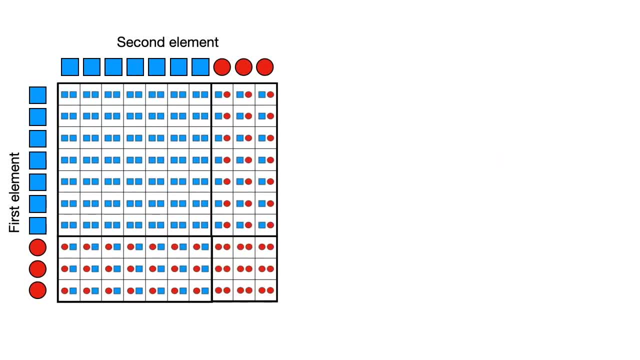 index. Let's quickly calculate it for the other data set. So in this data set I only have blue squares and red circles, And my probability that they're both blue squares is seven tenths squared. The probability that they're both red circles is three tenths squared And the probability that I 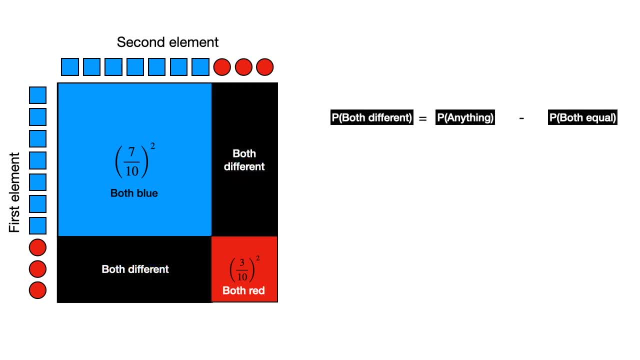 want that they're both different is the remaining area. So I do my math again: Probability of both different is probability of anything minus probability of both equal, which is one minus blue area minus red area, which is one minus seven tenths squared minus three tenths squared. 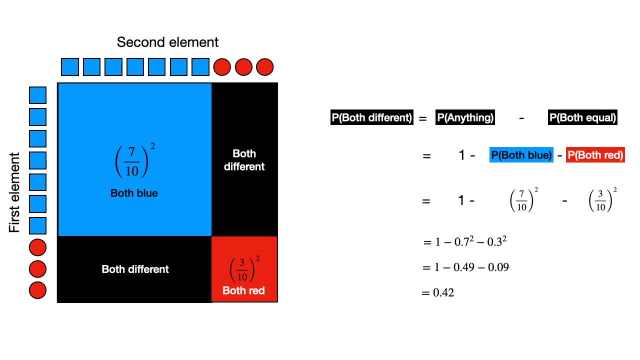 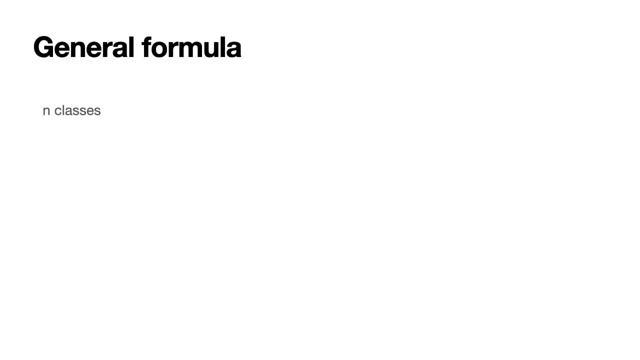 which is precisely 0.42.. So that's why I get the Gini index to be 0.42 for the second set. So the general formula: I'm going to have a set with n classes. Classes can be whatever And each class has a proportion. So the proportions are p1, p2, up to pn. So for the 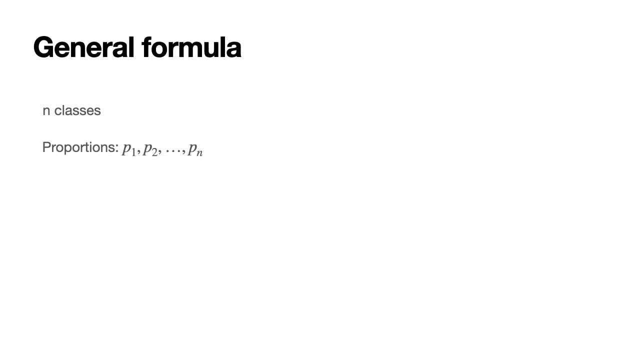 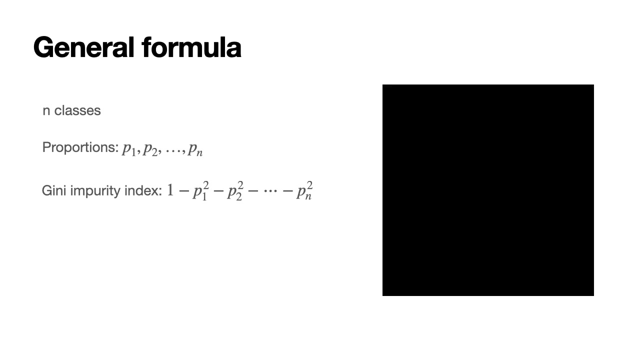 ith class, there's pi, a percentage of elements of that n class, And the Gini periodic index is simply one minus the sum of squares of those proportions. And the proof is the same. You have your square, which is of area one, and your smaller squares, each one for each one of the classes And the 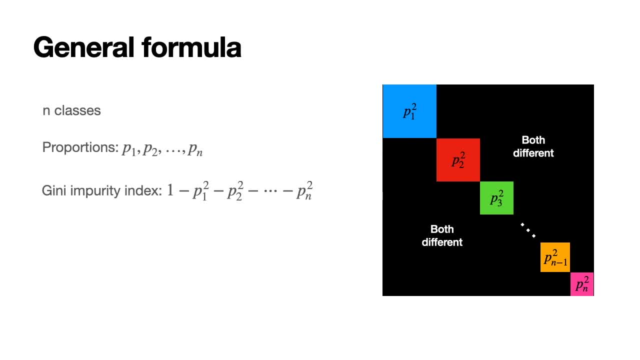 probability that the two elements that I pick are different are the black areas that are not corresponding to any of the color squares. So my probability of both different is Gini periodic index. My probability of anything is one And the probability of both equal is the sum of the areas of the 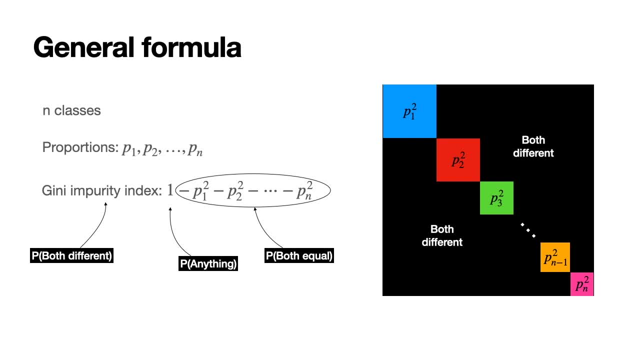 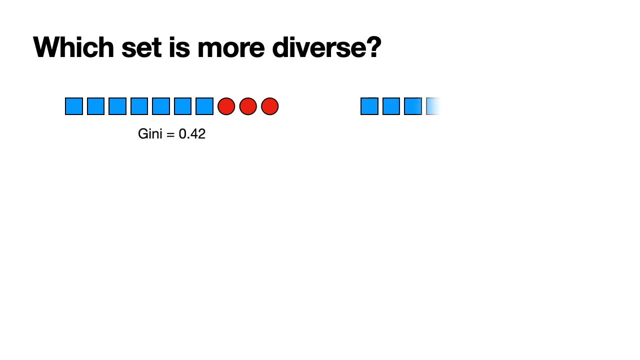 color square, which is the sum of pi squared from i, equals one to n. And now we go back to our data sets. The first one, as we calculated, has a Gini index of 0.42.. The second one, 0.7.. What about this one, the purely homogeneous data set? 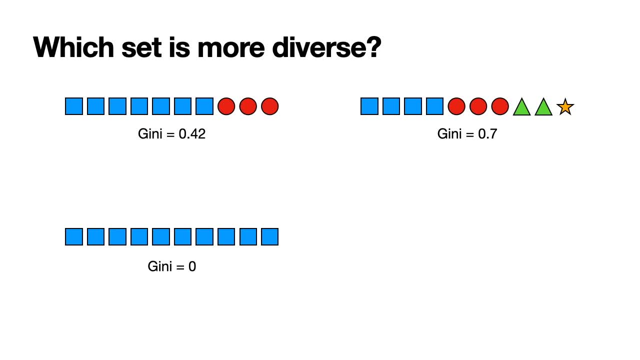 Well, that one has a Gini index of zero, And the reason is because every element is a blue square, So the proportion of blue squares is one, So it's one minus one squared, which is equal to zero. That's the Gini index. And what about the most diverse data set, one where 10 elements are. 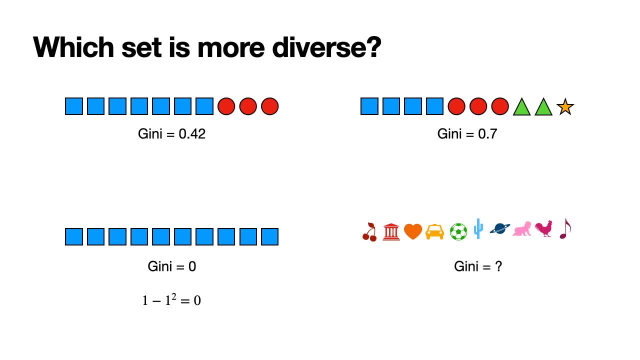 completely the same. What's the Gini index of this one? So I encourage you to pause the video and calculate it. And what I got for this data set is 0.9, because it's one minus 0.1 squared 10 times, And the reason is that each class appears one-tenth of the time. So this one gets.